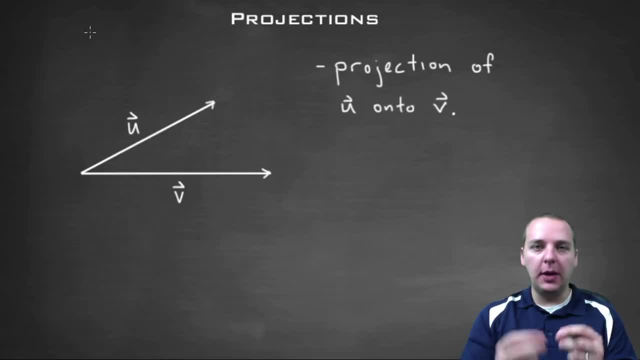 vector onto another vector. and how do you do it? pencil and paper, formula wise. So here's the basic idea: If you have a vector U and you have a vector V and you want to project U onto V, think of it almost like a shadow, so to speak. Meaning if V was the ground and 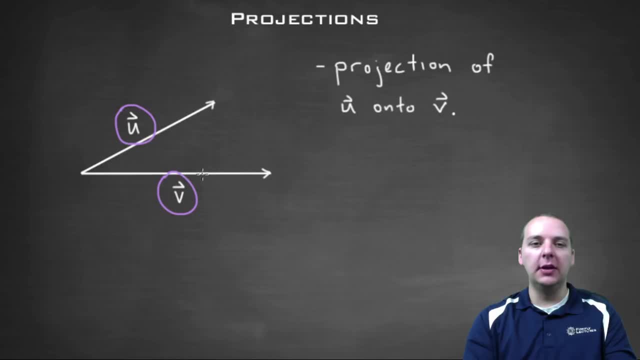 V is not always going to be horizontal, but let's assume that it is. Just for this example. if there was a light right here, do you notice how there would be a shadow that U leaves on that Okay V. So if you projected U onto V, it would wind up looking something kind of like this: 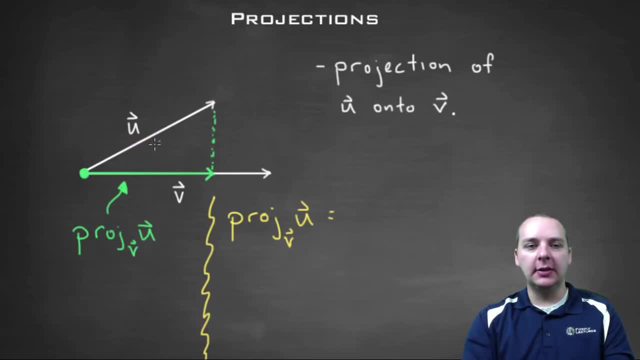 Let me get rid of all these purple lines. Uh, it looks something kind of like this: Uh, do you see the green vector? The green vector is what we call a projection. You're projecting U onto vector V. Notice that would be very different than projecting. 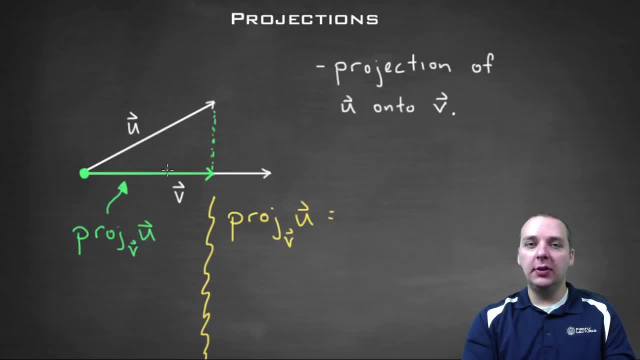 V onto U. So this green line, this green vector, is the guy we're going to try to find, And there's a formula for it that I'm going to give you right now. The first thing that I notice about the green projection vector is that it's in the same 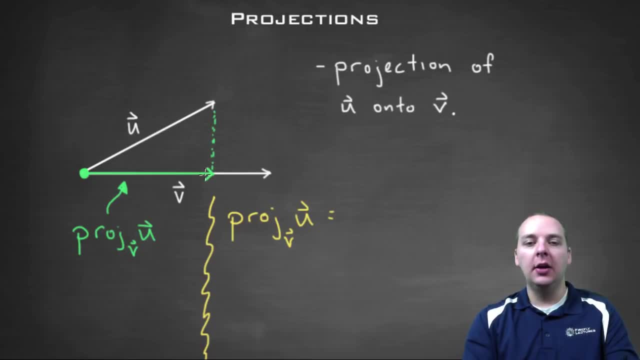 direction as V, since it was projected onto V, Which means it's simply going to be some scalar multiple of vector V. I didn't need anybody's help to determine that much. Uh, it's going to be either shorter or longer than V. uh, depending on how long U is. 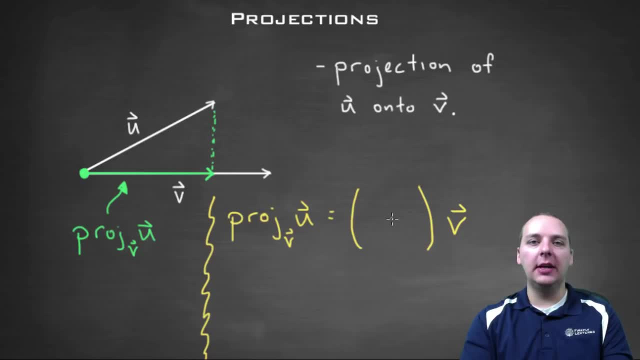 Uh, now the, the, what the scalar Vector is, is a little less intuitive. Um, let me give it to you. It's U dot V divided by the magnitude of V squared. So you might want to jot this formula down and commit it to memory, but this is your. 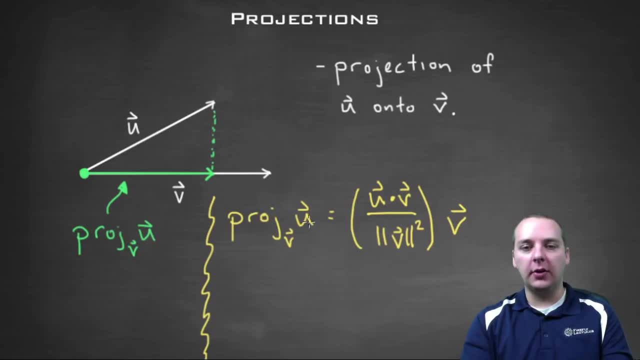 formula for a projection, projecting one vector onto another vector. So you uh notice, the dot product is a scalar and the norm is a scalar. So a scalar Divided by a scalar is another scalar, And so you're going to scale V by a certain amount. 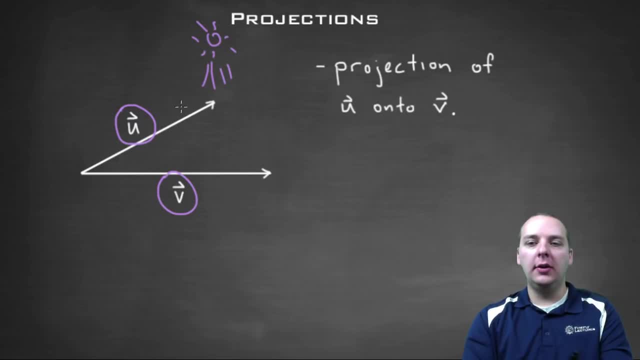 onto v. So if you projected u onto v, it would wind up looking something kind of like this: Let me get rid of all these purple lines. It looks something kind of like this: Do you see the green vector? The green vector is what we call a projection. You're projecting. 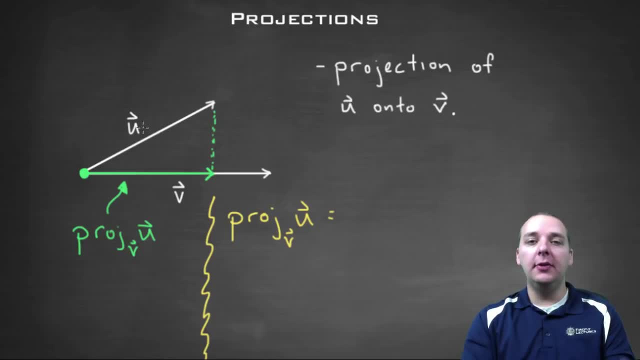 u onto vector v. Notice that will be very different than projecting v onto u. So this green line, this green vector, is the guy we are going to try to find and there's a formula, formula for it that I�m going to give you right now. The first thing that I notice about 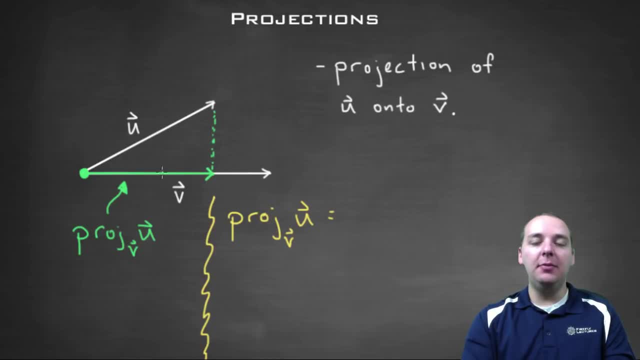 the green projection vector is that it�s in the same direction as V, since it was projected onto V, Which means it�s simply going to be some scalar multiple of vector V. I didn�t need anybody�s help to determine that much. It�s going to be either shorter or longer. 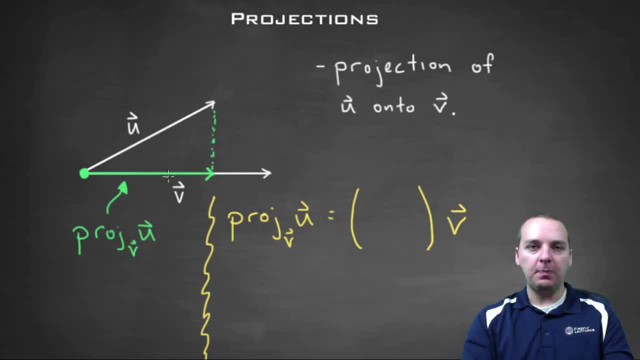 than V, depending on how long U is. Now, what the scalar is is a little less intuitive. Let me give it to you. It�s U dot V divided by the magnitude of V squared. So you might want to jot this formula down and commit it to memory. But this is your formula for a. 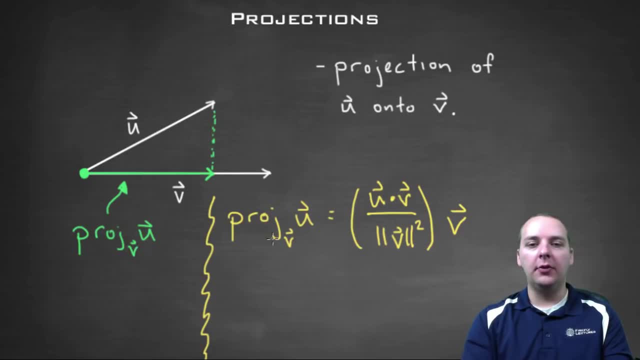 projection, Projecting one vector onto another vector. So notice: the dot product is a scalar and the norm is a scalar. So a scalar divided by a scalar is another scalar, And so you�re going to scale V by a certain amount And 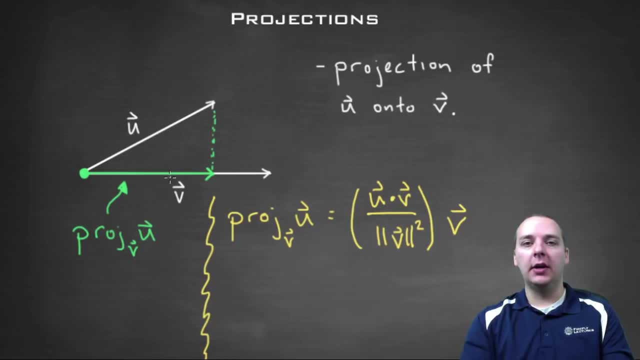 this happens to be just the right amount to give you this green vector right here And again. let me reiterate: we�ll talk about why this is important towards the end of this video. Alright, let me reorient this picture here and let�s see if you can find just. 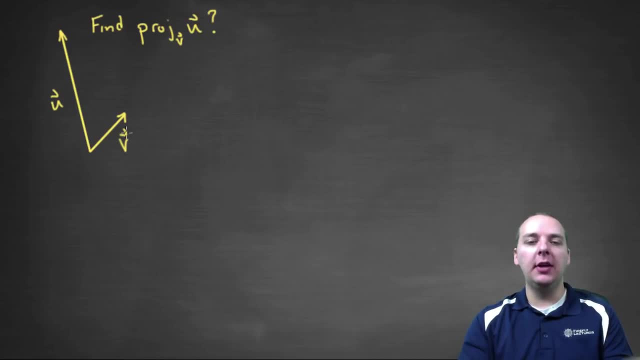 what the projection would look like. So here�s U, here�s V. I�ve kind of flipped them all around because they�re not always going to be pretty and nice and flat and that sort of thing. Can you visualize what the projection of U onto V would look like, So in your mind? 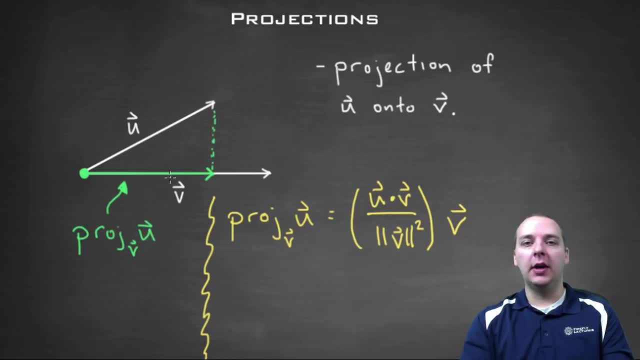 And this happens to be just the right amount to give you this green vector right here And again. let me reiterate: we'll talk about why this is important towards the end of this video. All right? Um, let me reorient this picture here and let's see if you can find what, just what? 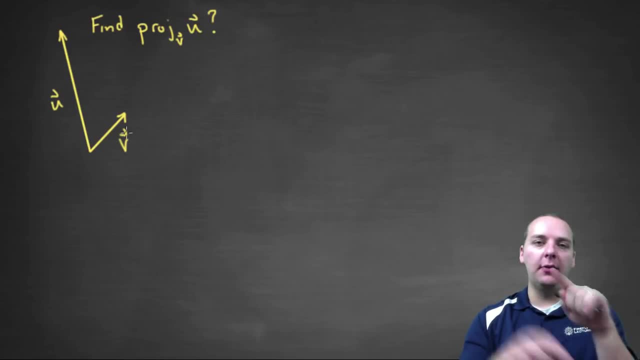 the projection would look like. So here's U, here's V. I've kind of flipped them all around, cause they're not always going to be pretty and nice and flat and that sort of thing. Can you visualize what, what the projection of U onto V would look like? 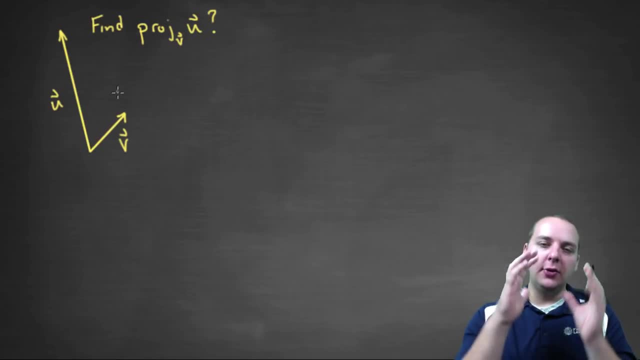 So in your mind, here's what you do: You either tilt your head or you think you think of V as being the ground and then think of there being like a sun at 12 o'clock noon shining directly onto the ground. So here's: the sun is shining onto the ground because the ground is is kind of tilted this way. 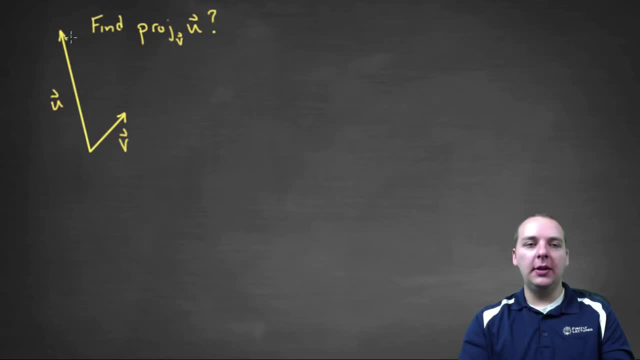 And I think I can see it. Uh, this guy would leave a shadow, something kind of like this. So here this green vector that I'm drawing right here. that would be the projection of U on to V. Now notice, in this example the projection is longer than V, and that's okay. 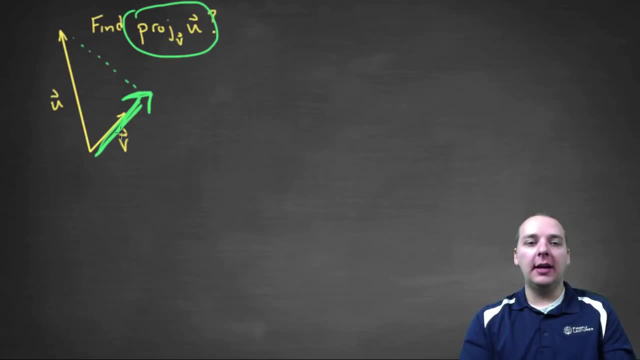 And the other example. the projection was shorter than V, but nevertheless it's going to be some scalar multiple of V, So Hopefully you got the same vector that I did here. All right, Now, that's all well and good, but like what might this possibly be used for? 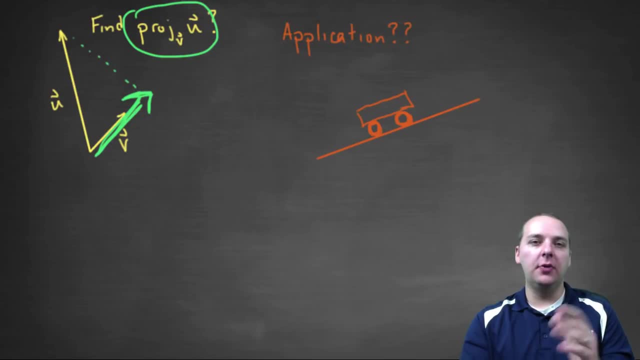 Well, let's close out this video just talking about, uh, just a very common example that uses projections. A lot of these examples will have something: a truck, a boat, a box, a something sitting on a hill. Now, obviously, due to gravity, there's a force vector that's applied to this object. 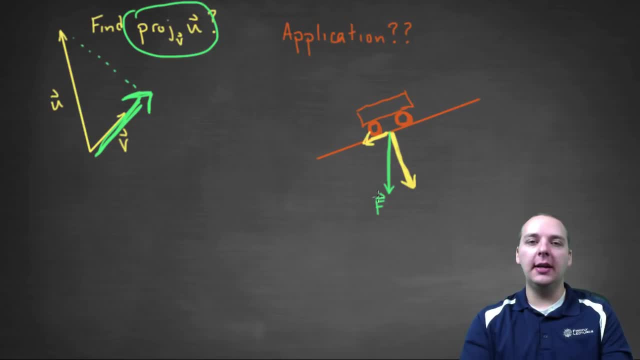 Okay, On the hill and this force vector goes straight down. But a very common question that we see, uh, a lot dealing with these projections is how much force would be required to hold this box up on the hill. So if this, you know, if this box on the wheels weighed 200 pounds, it obviously wouldn't. 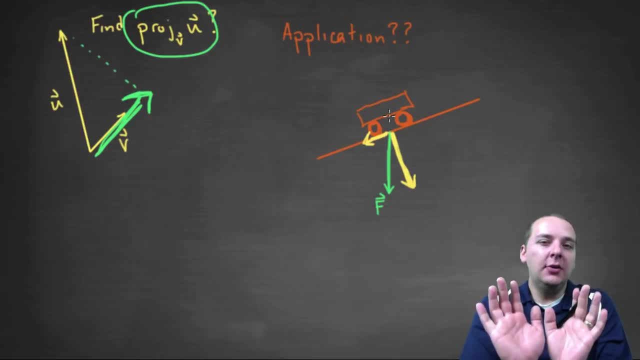 take 200 pounds to hold it up on the hill, because the hill is helping you a little bit. The steeper, the hill, yeah, the harder it would be. But, um, The flatter the angle, the easier it'll be. 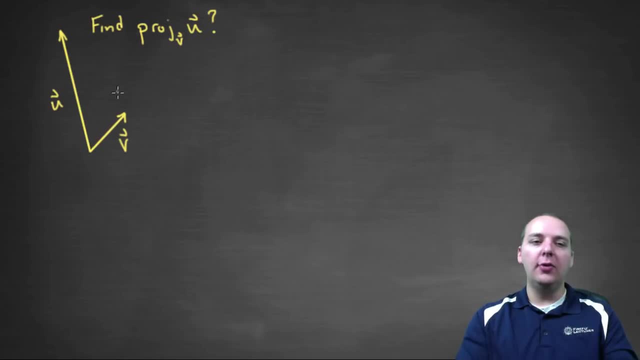 here�s what you do: You either tilt your head or you think you think of V as being the ground and then think of there being, like, a sun at 12 o�clock noon shining directly onto the ground. So here�s the sun shining onto the ground, because the ground is kind of tilted. this 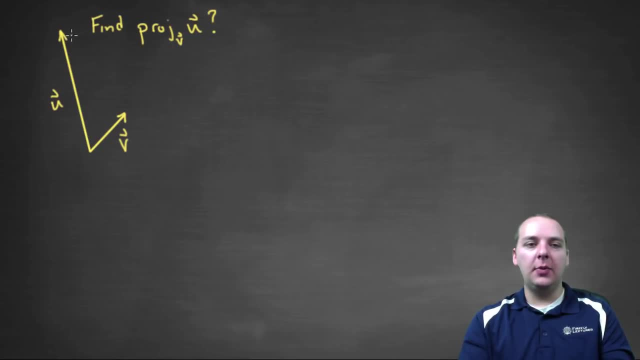 way, and I think I can see it, This guy would leave a shadow, something kind of like this. So here this green vector that I�m drawing right here. that would be the projection of U onto V. Now notice, in this example the projection is longer than V, and that�s okay. And the 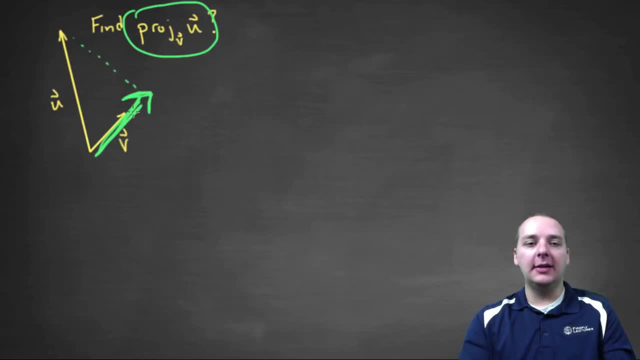 other example, the projection was shorter than V, But never mind. Nevertheless, it�s going to be some scalar multiple of V, So hopefully you got the same vector that I did here. Alright, now that�s all well and good, but like what might this possibly be used for? 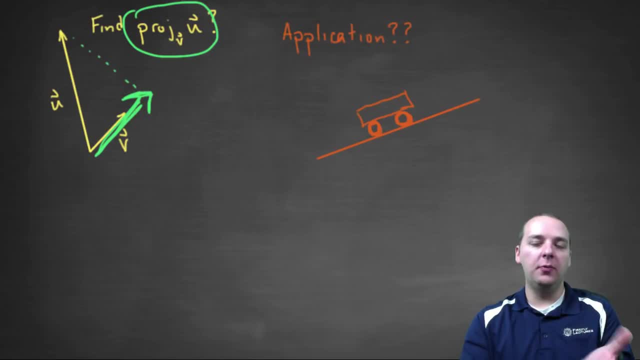 Well, let�s close out this video just talking about just a very common example that uses projections. A lot of these examples will have something: a truck, a boat, a box, a, something sitting on a hill. Now, obviously, due to gravity, there�s a force vector that�s applied to this object on 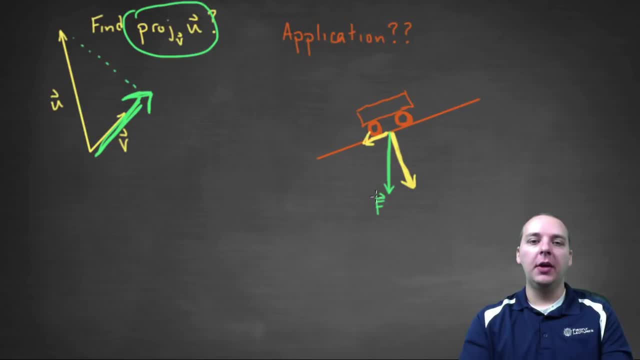 the hill and this force vector goes straight down. But a very common question that we see a lot dealing with these projections is how much force would be required to hold this box up on the hill. So if this you know, if this box on the wheels weighed 200 pounds, it obviously wouldn�t. 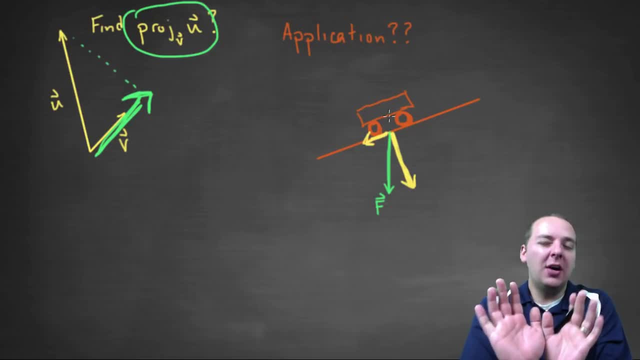 take 200 pounds to hold it up on the hill, Because the hill�s helping you a lot. The steeper the hill, yeah, the harder it would be, But the flatter the angle, the easier it will be. So what�s happening is this force vector. if you project it onto the hill, like if you 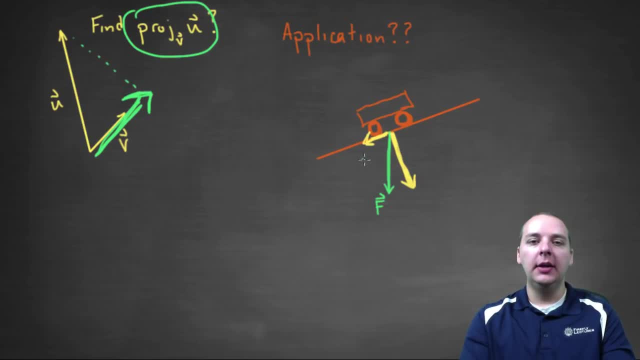 have a vector here that�s in the same slope as the hill, then you�re just getting part of the force. So notice however long this vector is. that�s how much force you�re going to have to apply in the other direction.